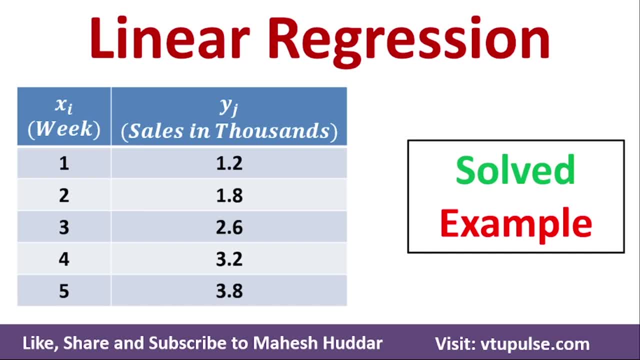 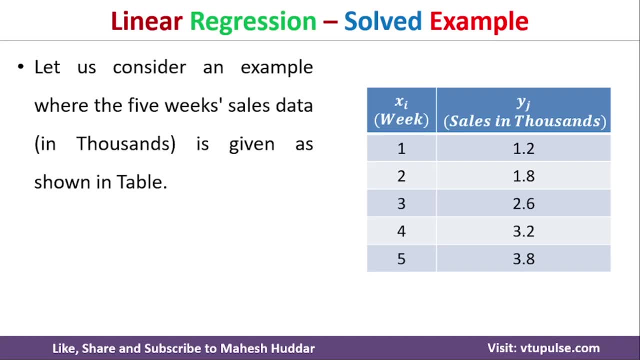 Welcome back. In this video I will discuss linear regression algorithm with a simple, solved example. In this case, we have been given an example with five weeks sales data. Given this particular data set, we need to apply the linear regression algorithm and then we need to predict. 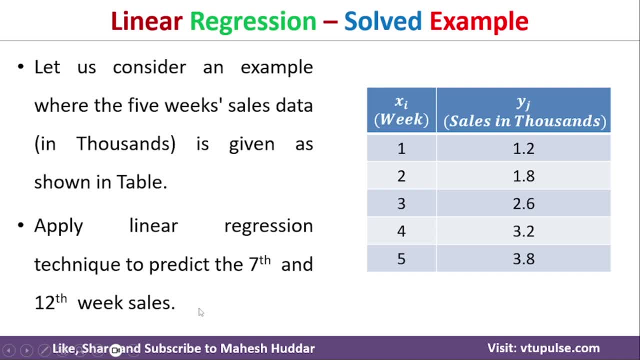 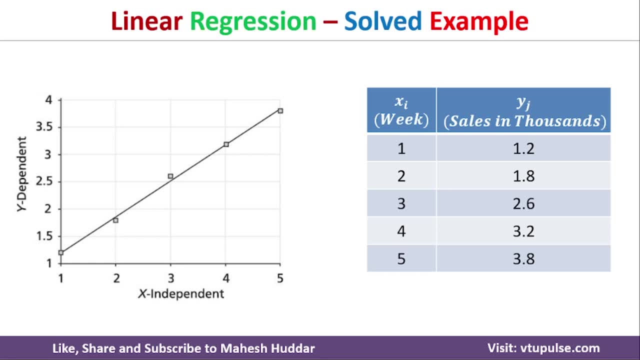 the sales in seventh and twelfth week over here In linear regression algorithm. first we will plot the independent variable against the dependent variable. In this example, x is an independent variable and y is the dependent variable. All these five points are plotted over here. 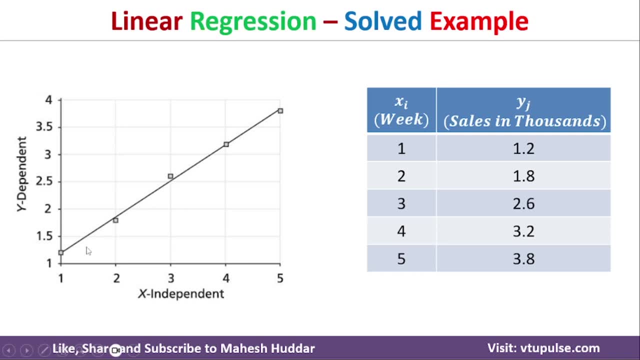 The goal of linear regression is to find a straight line which will fit this particular given data set perfectly. The equation for this particular line looks something like this: y is equivalent to a0 plus a1x plus e, where e is the error in this case. 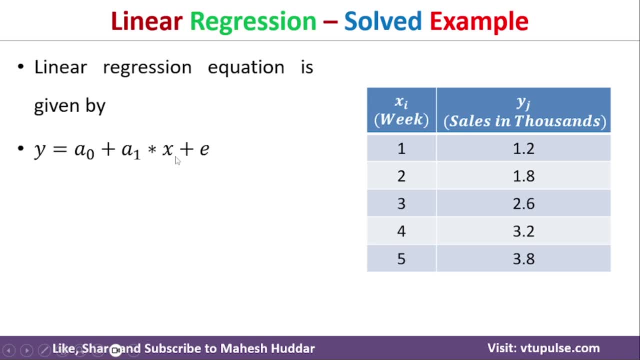 a0 is the intercept and e1 is a coefficient of independent variable, That is x here. Now the next question comes in front of us: How to calculate this a0 and e1 in this case. First we will understand how to calculate the value of a1. 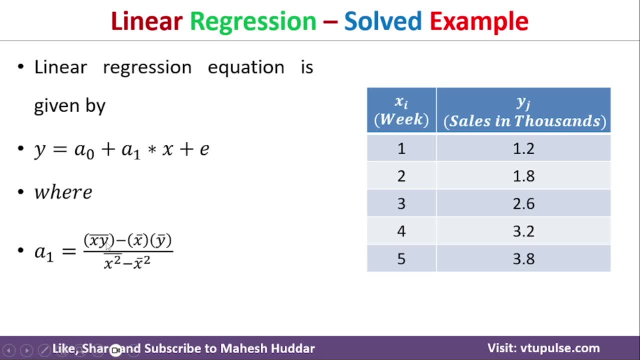 a1 is always equivalent to first. we need to calculate xy, that is, the multiplication of x and y, and then we need to take the mean of this column Minus. we need to calculate the mean of x and then the mean of y over here divided by first. we need to calculate x square and then we need to calculate its mean. 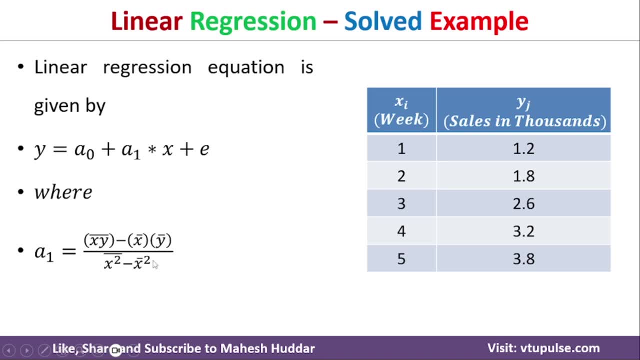 minus the mean of x, x square over here. once you calculate the value of a1, now we can calculate the value of a0. a0 is equivalent to mean of y minus a1. that is already calculated over here. multiplied by x bar, that is mean of x over here. so we know the value of x, we know the value of y. 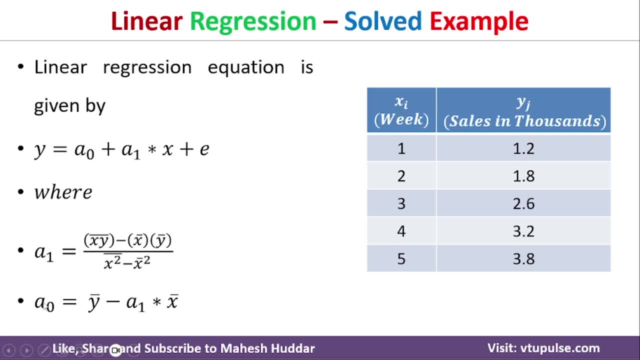 we need to calculate all these particular parameters. then we will be able to calculate a1 and a0. once you calculate the value of a1 and a0, we will get the linear regression equation here. once you know the linear regression equation, we can calculate the value of dependent variable that. 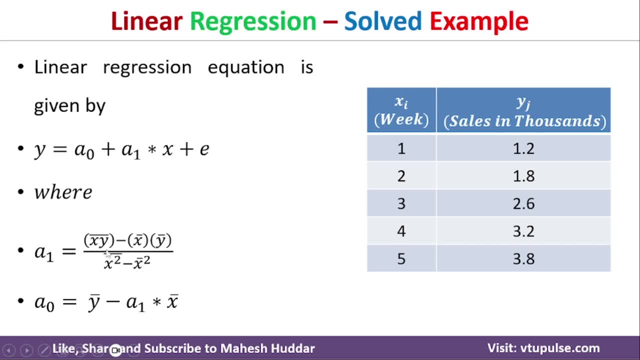 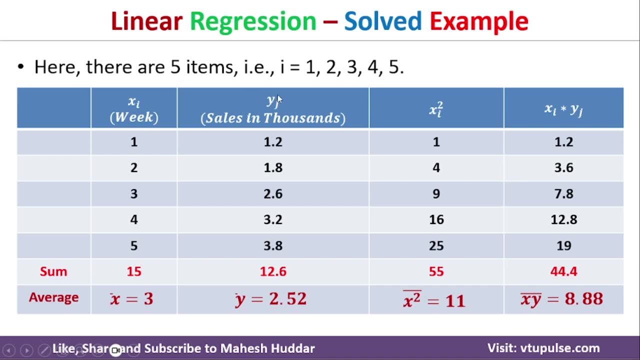 is y, given this particular x over here. so first we will try to calculate all these particular parameters. so the, given this particular x and y, we need to know the mean of x. so we will calculate the sum of all these particular values. we will get 15, 15 divided by 5, which is nothing but the mean of this particular x. 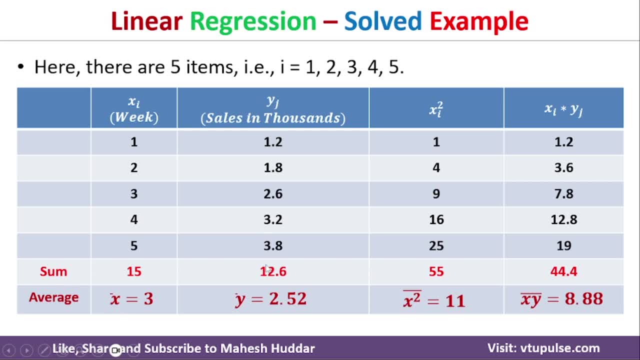 similarly the y column. we will add all these things, we will get 12.6 divided by 5. that is nothing but the mean of y over here. first we will calculate x square, that is nothing but 1 into 1, that is 1, 2 square is 4, 3 square is 9, and so on. so once you calculate all these things, we will. 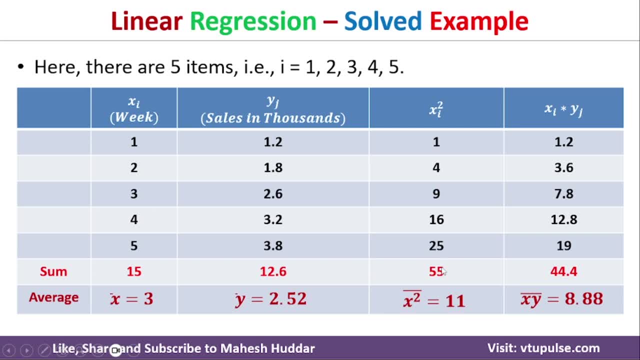 calculate the sum of all these things, which is nothing but 55. the mean of this particular 55 is 55 divided by 5, that is nothing but 11. over here, first we will calculate x, y, that is x into y. 1 into 1.2, that is 1.2, 2 into 1.8, that is nothing but 3.6, and so on. 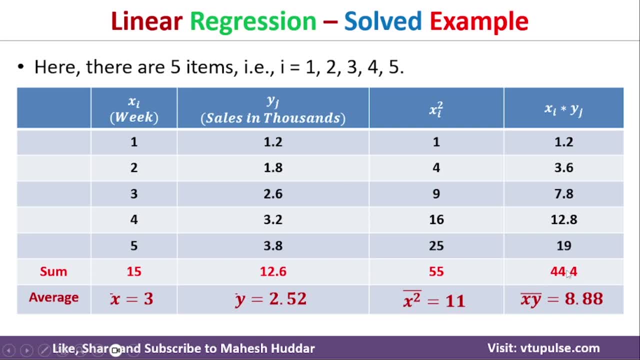 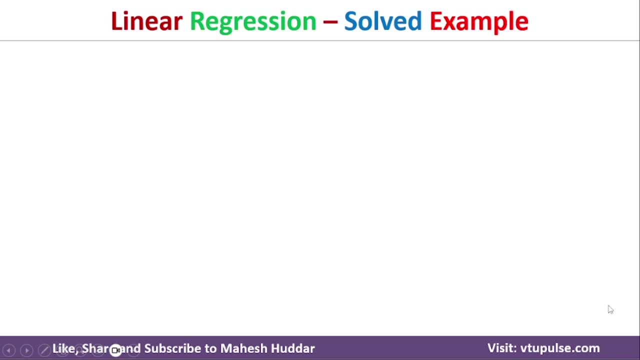 we will get 44.4 here. 44.4 divided by 5, that is nothing but the mean of x, y over here, which is equivalent to 8.88 in this case. once you calculate these particular parameters, we will put this particular parameters in a1 equation. 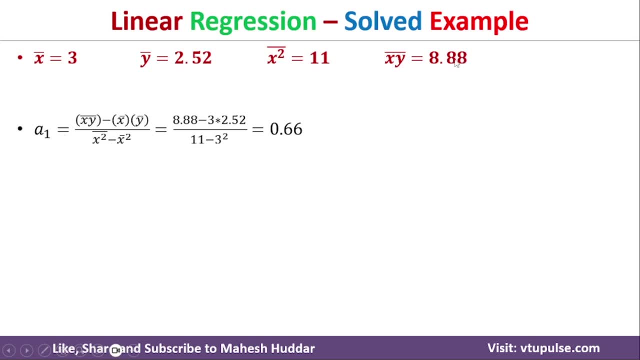 a1 is equivalent to x y bar. that is already calculated. here x bar is calculated. y bar is calculated divided by x square bar. we have already calculated here. x bar is known to us. its square is calc. we can easily calculate it. so we will put all those particular values. 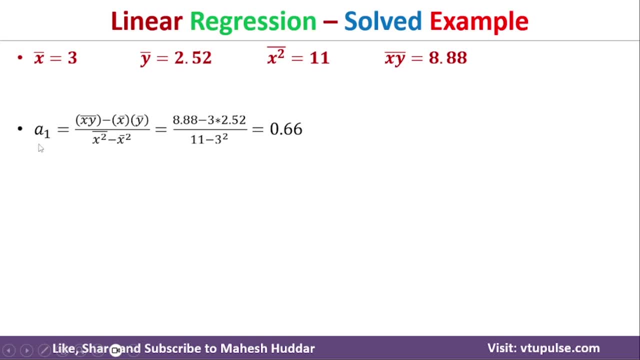 we will get the value 0.66 as a1 in this case. so once you calculate the value of a1, we need to calculate the value of a0. a0 is equivalent to y bar minus a1, x bar. so we need to put all these particular values. we will get 0.54 in this case. once you know the 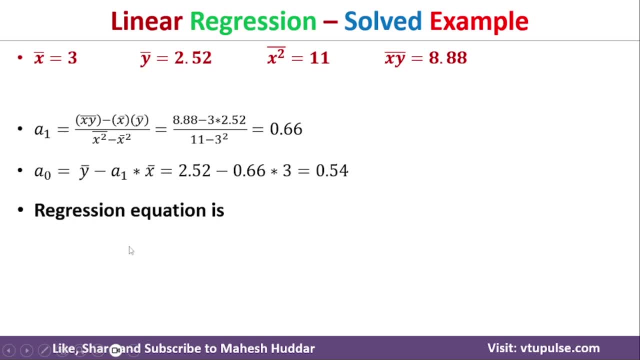 value of a0 and a1. we know the equation for linear regression, that is: y is equivalent to a0 plus a1. x. a0 is known to us, a1 is known to us. the linear regression equation will become: y is equivalent to 0.54 plus 0.66 multiplied by x. over here, once you get the equation for linear regression.